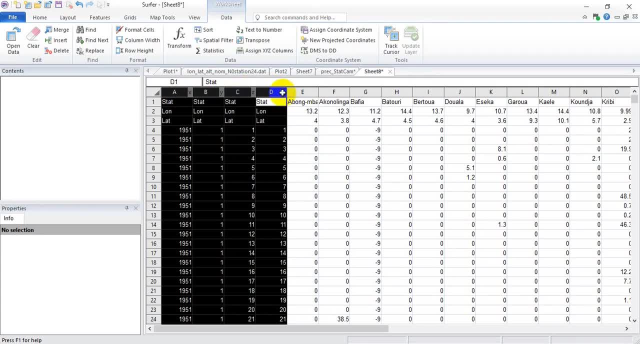 day and then click on the date of the month, And then I will come and put the Wallah: This tree. I will copy. Okay, This is the second time And then I will come back here. Okay, Now I will open the next thing. 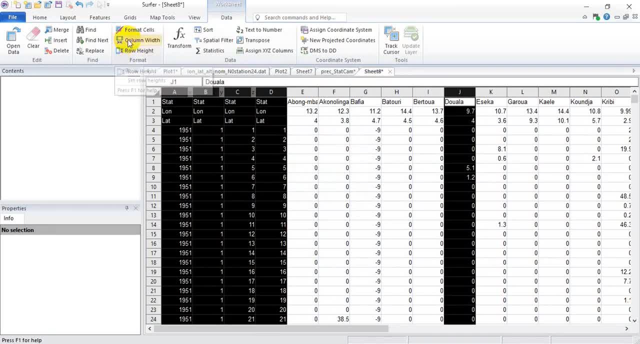 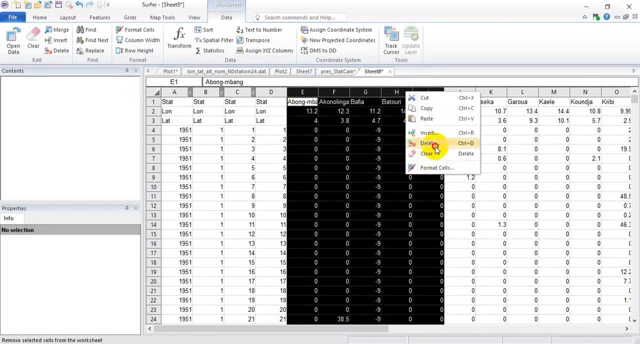 Okay, I will do the same for this one. I will put this: See, I just copied the same piece of data into my new sheet. Okay, Now I am going to my new sheet. Now I have my new sheet. So I will go to my new sheet and I will paste this here. 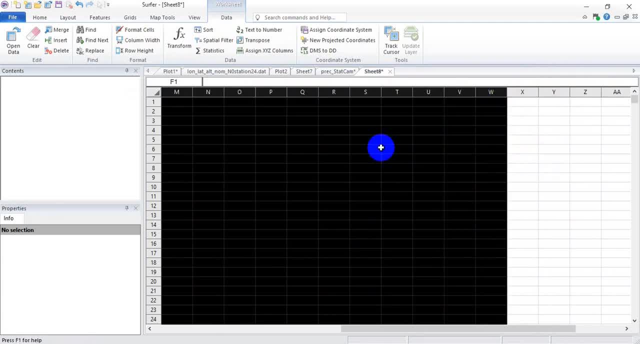 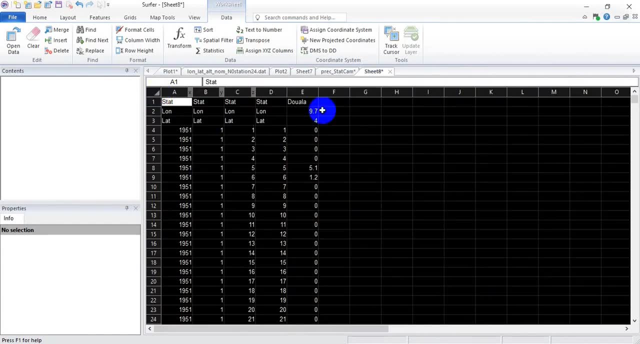 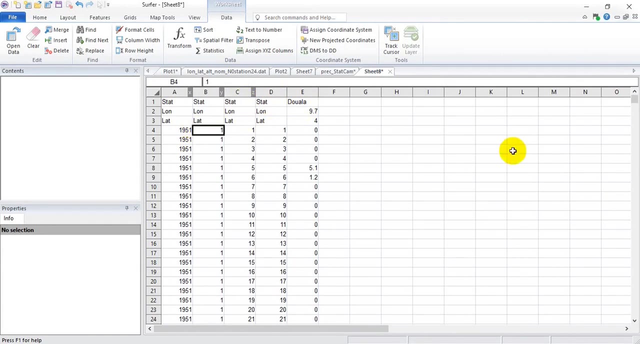 Okay, Copy. Come to my sheet. Come to a new sheet. Copy that still. Just delete this And then delete the rest, Because I already have them duplicated. So this is our worksheet, What we need. We need here wallah, and we need the years. so the next thing we need to do is to get a mean for 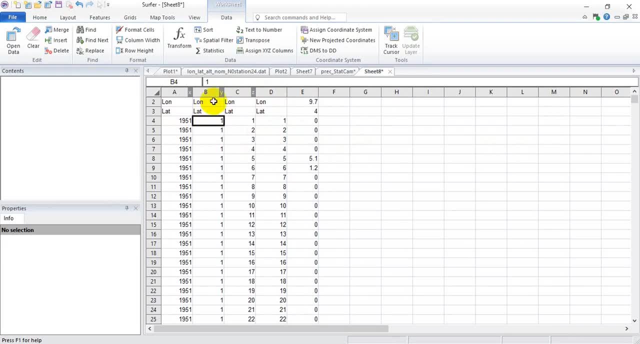 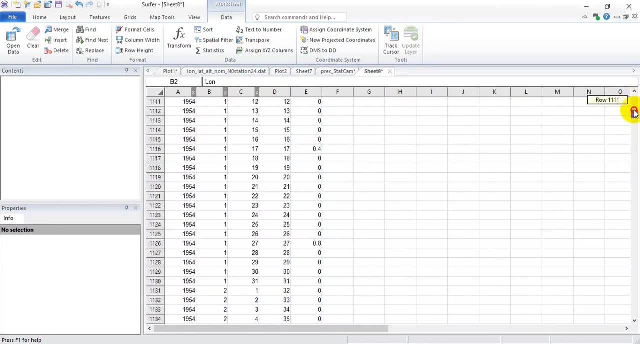 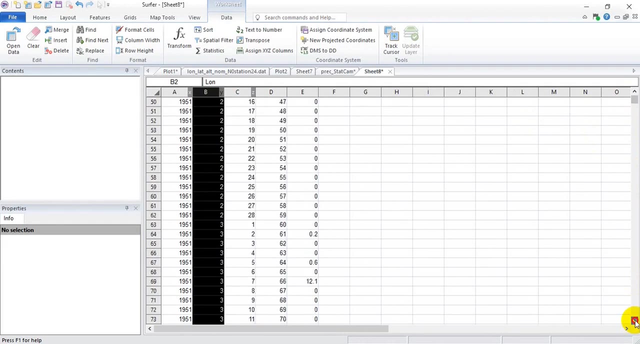 the month and the Monday mean means who do? who sought this column of? you see how different months of the year, 1 to 12, as you can see different ones, 1, 2, 3, 4, for all the years. so what we do is we do perform a sought to perform the sorry. 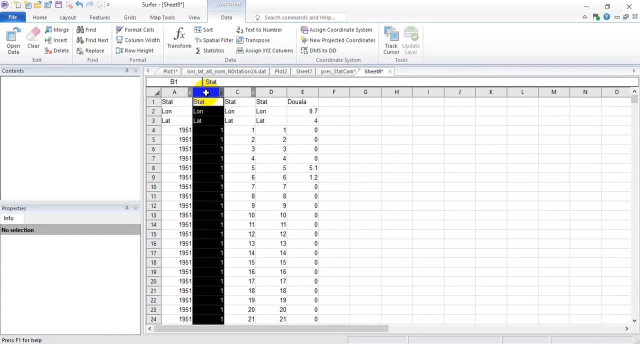 right click on the top, we click on here, you click on sought that. I sought by ascending or descending. ascending is from 1 to 12 and descend is from 12 to 1, so I'll go by so by ascending and I click OK. so I have not my statistics. 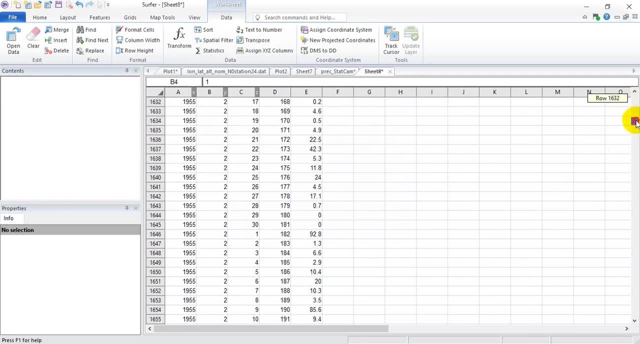 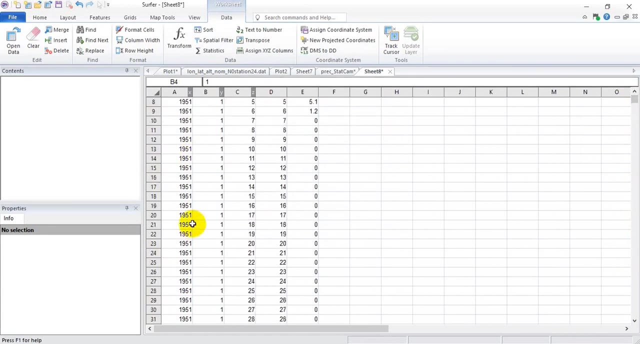 if you look now, I've ordered for the first month of each year, after the second month, third, fourth, fifth. it has been sorted out already. so what we need to do next is to scroll down to the first month of each year and we need to scroll down to the end date of the first month. 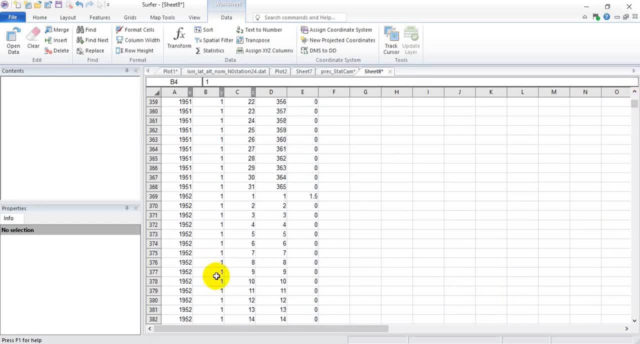 screwed on to the filter of the first month. maybe time-consuming rule- you just scroll down to the day of the first month, but it is not allowed. yes, this must be in number three because currently all dates can be one of two random dates of the month and for this we need to see how many dates it is. 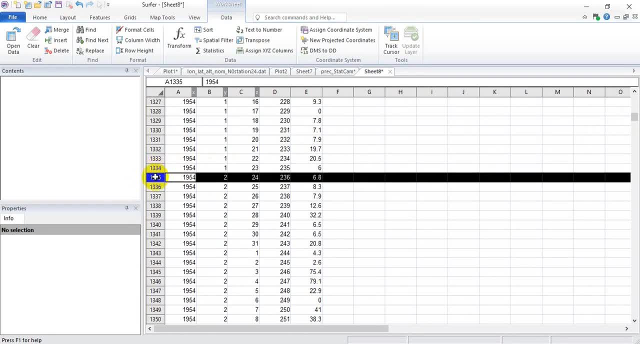 three months, the あ two next coming months. so what they are? the third month. if you click first month, atomized it. the second month and the fourth month is the date where lockdowns happen. the third month and she goes through it one by one: the. 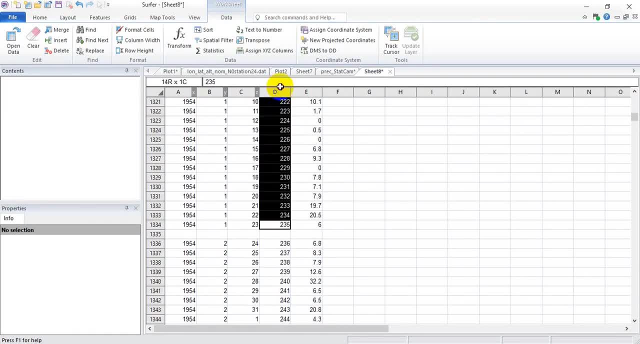 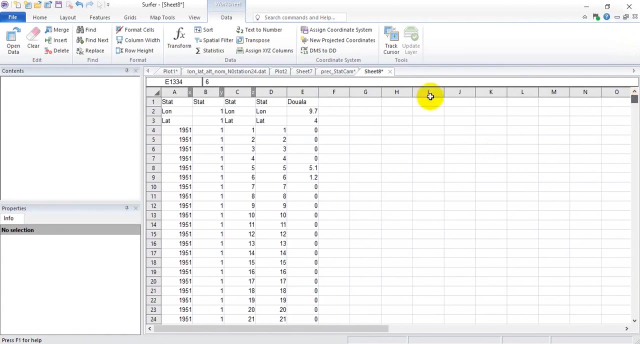 come to this and you select: oh sorry, come to the another info. or, better still, you click here, then you come, you come, you click on, you press the shift button, I click on this, automatically selected. you go to statistics and mean mean standard error would only stand at the. 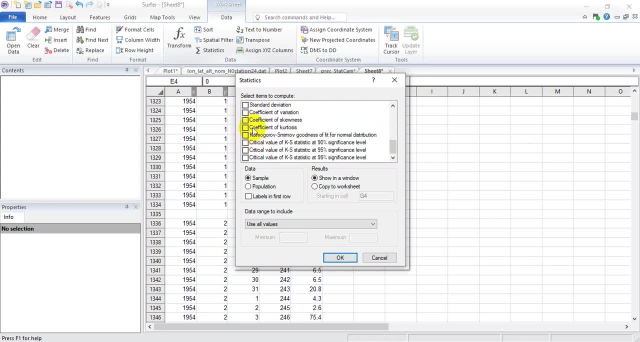 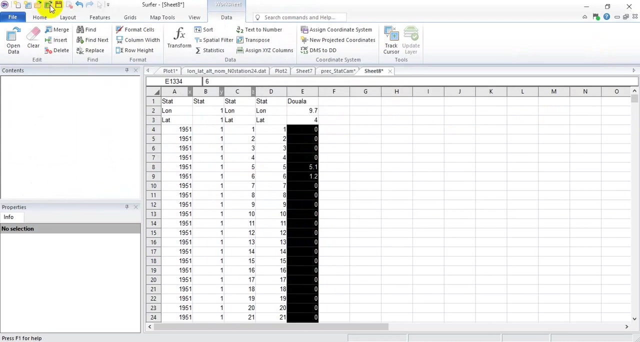 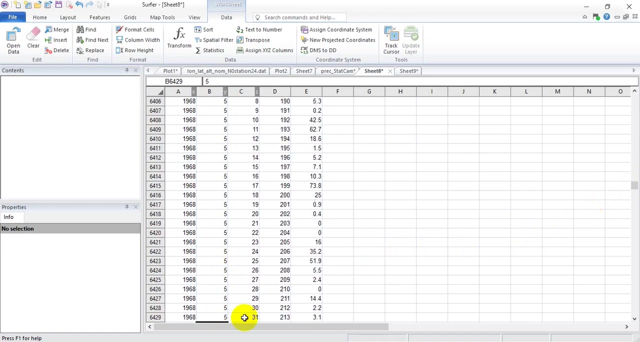 wrong subdivision. we need it. so we have this one. we copy: close it in your worksheet. you pissed, huh. yeah, yeah, yeah, yeah, I'm using the arrow key. so insert the top instead between six-and-five. you do so to reach the end. you use the screw, you screw down and you see seven. you click on seven and then you go up with arrow key. 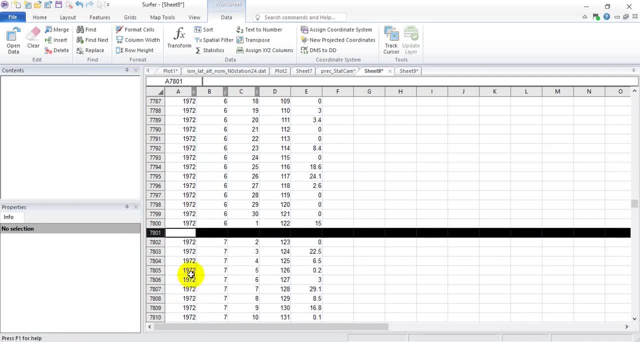 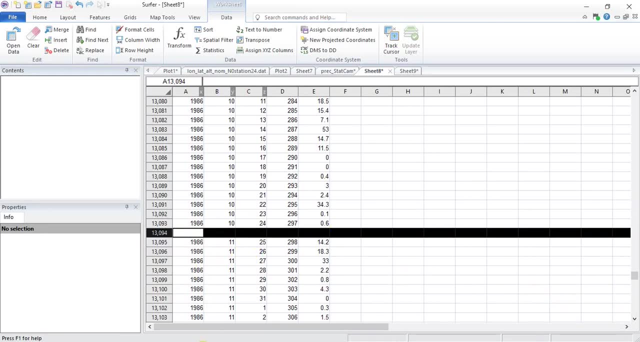 so you meet this line, just all the first column seven you do on inside the break. that's a break, you go down, okay. so once we have all the uh, call the interface. we then now select: just go to like for 12 to calculate the mean for 12.. 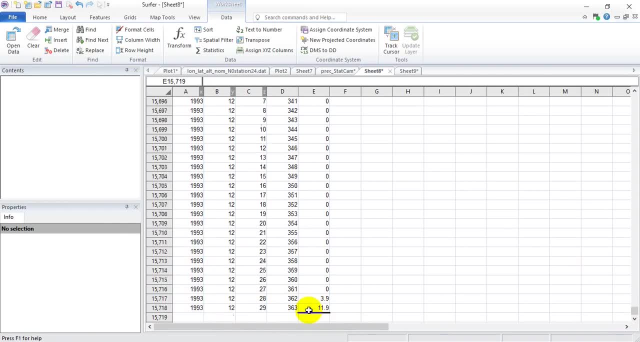 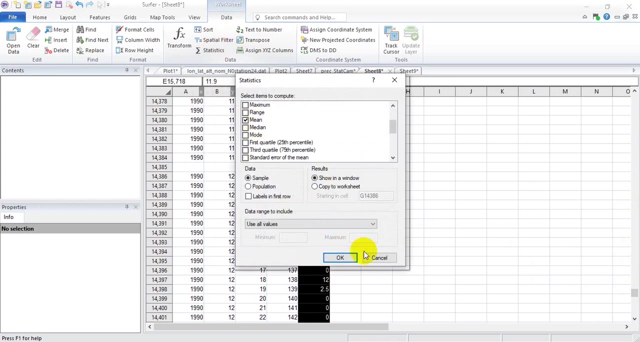 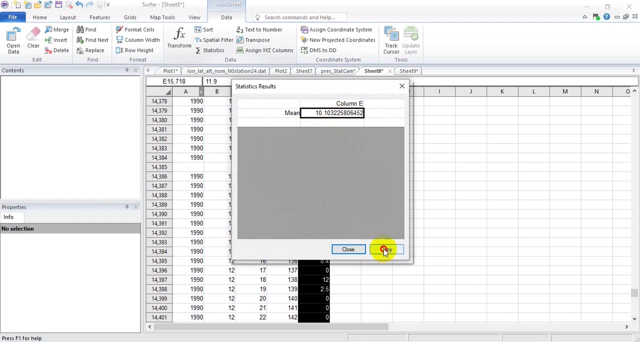 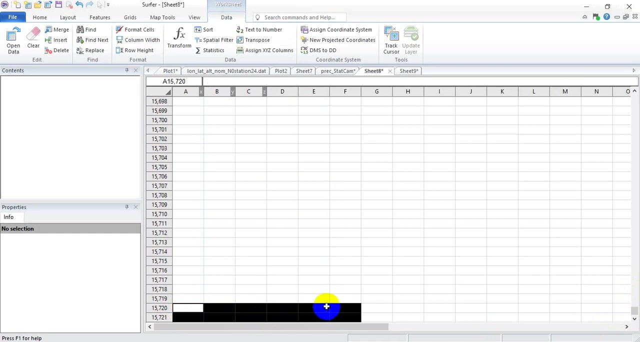 okay, to calculate the mean for 12. we just do this. so what i do is click here, shift, shift, shift, and i click here and i come to statistics and then okay, because means already selected. okay, okay, yeah, shift. this one's on the study, it is more space. 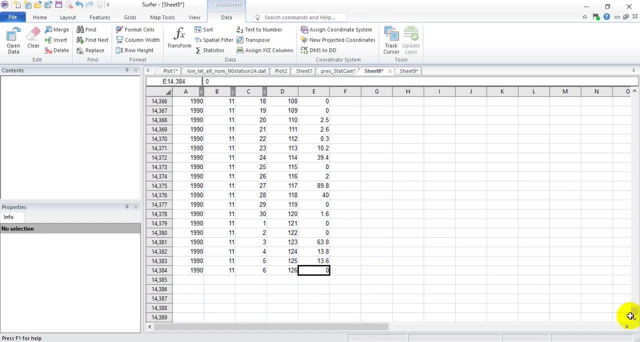 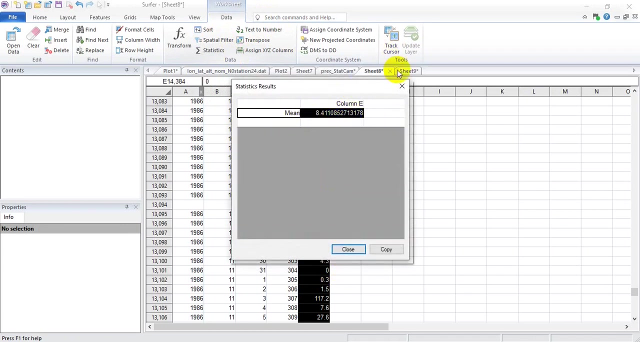 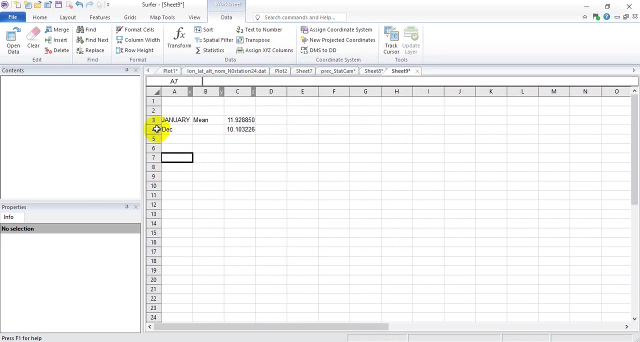 oh yeah, click, shift, shift, click here, let's go to statistics. okay, copy, copy, close, get to the sheet. Thank you, I'm going to control X: January, February, March, April, May, October, September, October, November, December. Then I come back to the sheet. 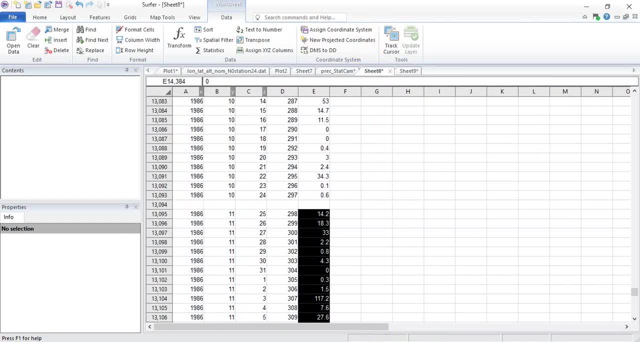 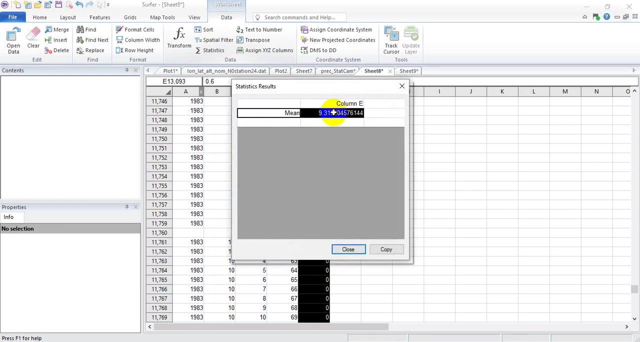 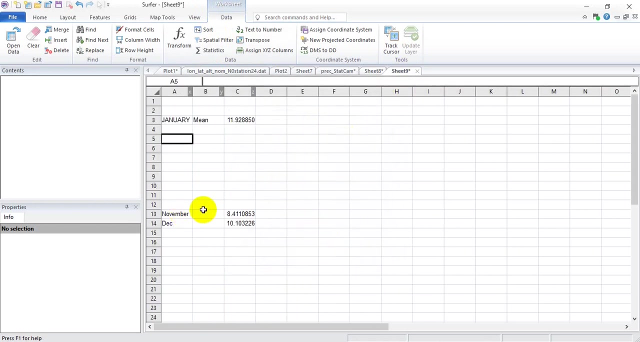 I just do. my hand is still on shift, I use the arrow key and I delete. I just delete. So it is my workspace. I don't want, I know shit. Statistics- Okay, Close. Go to the sheet. Okay. 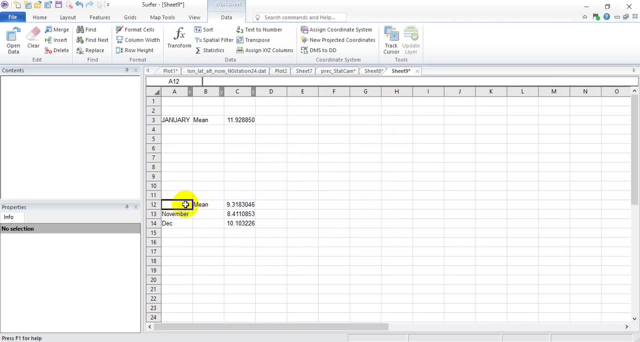 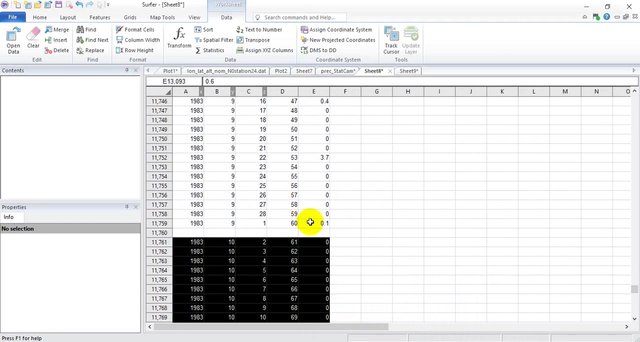 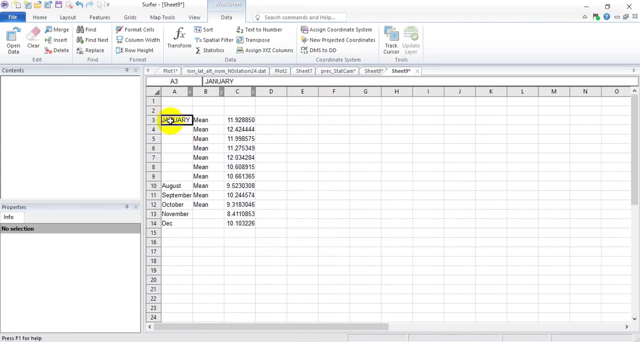 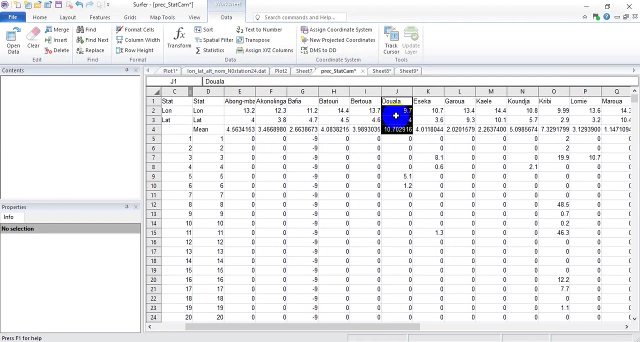 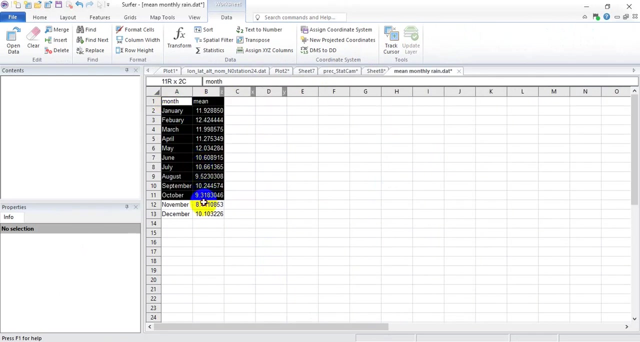